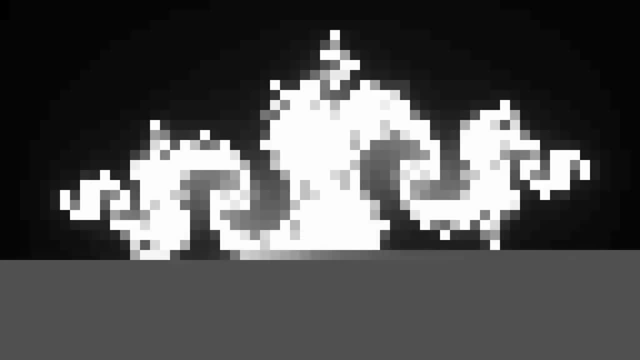 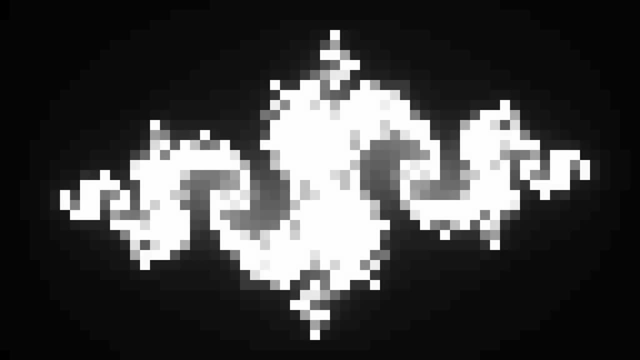 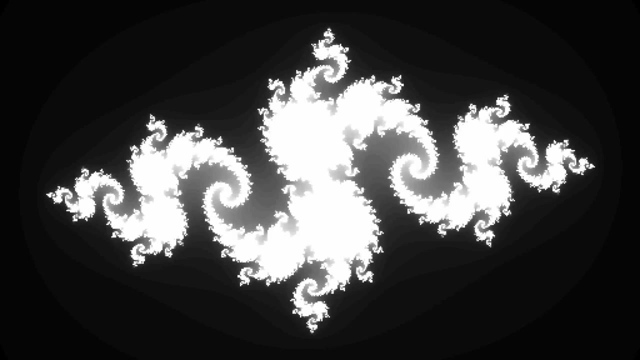 The result isn't very pretty. at this level of resolution, let's increase the number of pixels. We already have a high quality fractal. However, because we use the iteration count, which is an integer, to colorize pixels, the resulting image isn't very smooth. 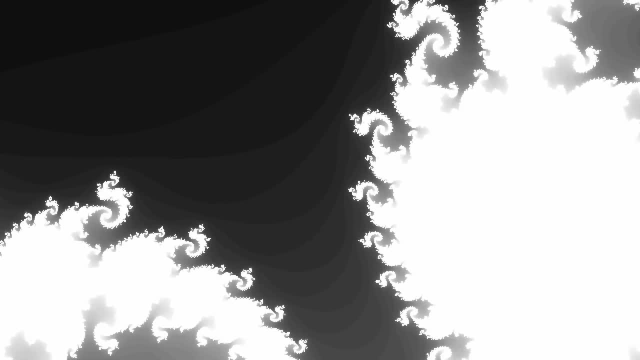 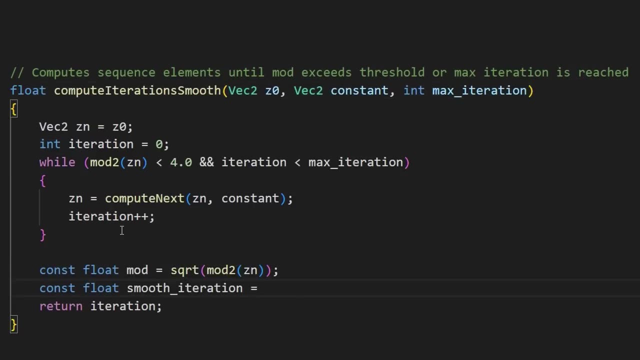 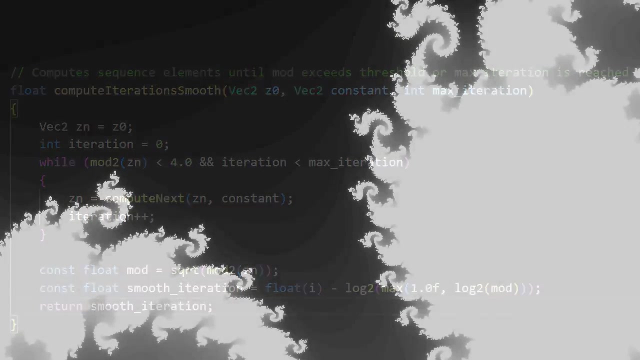 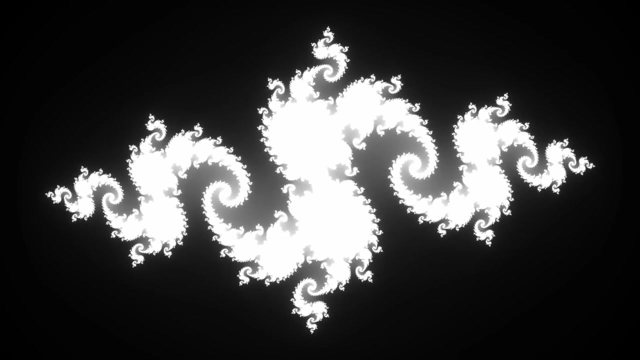 There is a simple fix for this. Instead of using the row integer value of the iteration count, we can apply this operation and return the float value. This is much cleaner, But we can see that pixels are quickly saturated because for a lot of them, 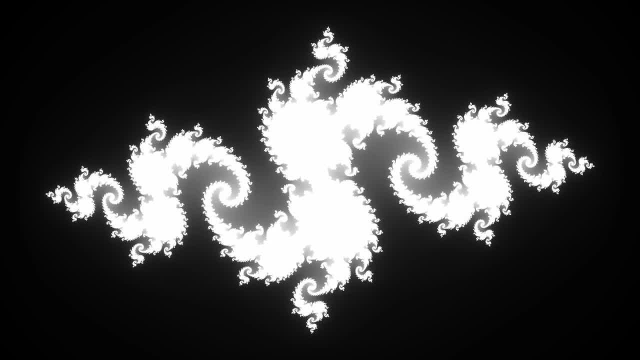 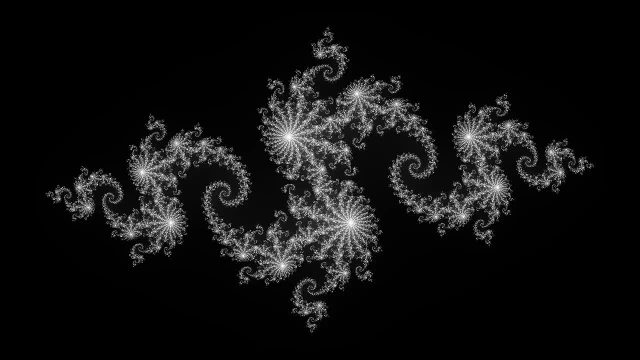 we reach the threshold of 50 while iterating on the sequence. To reveal more details of our fractal, we can simply increase the maximum number of iterations. Here I increased it to 500.. I am using the CPU to perform the rendering. 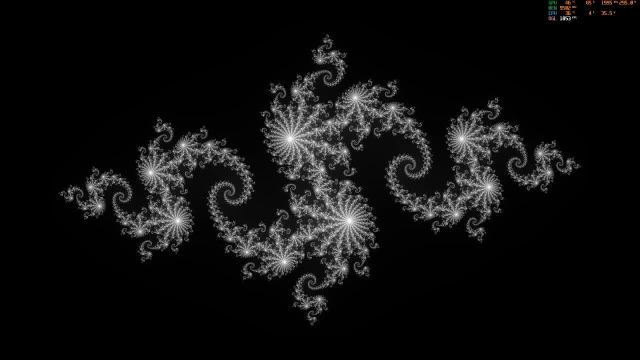 It could also be done with the GPU, and very easily. This is close to an hello world for shaders. Performance is also excellent, As you can see. the rendering is very smooth. The rendering is very smooth, As expected, Since this is the perfect use case for a graphic card. 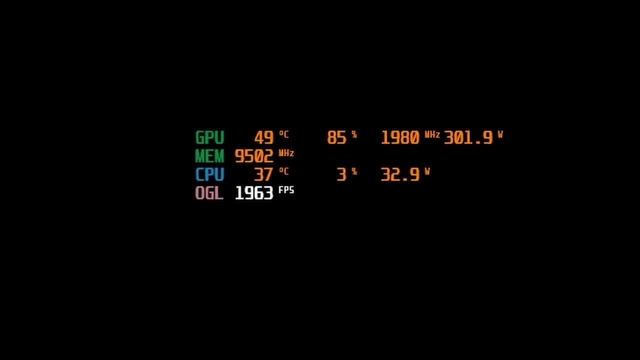 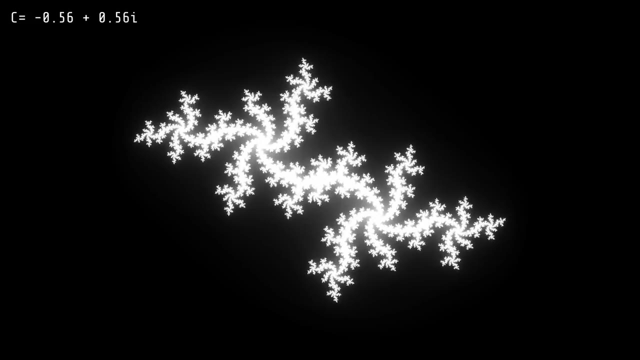 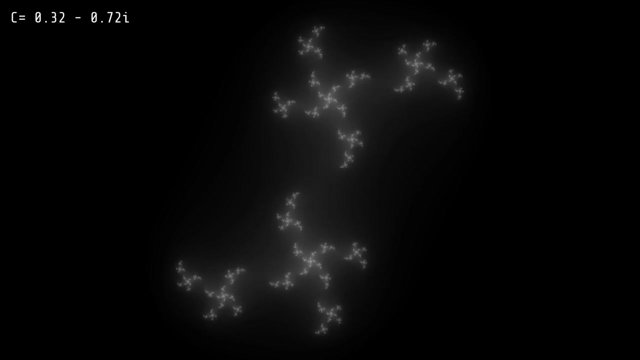 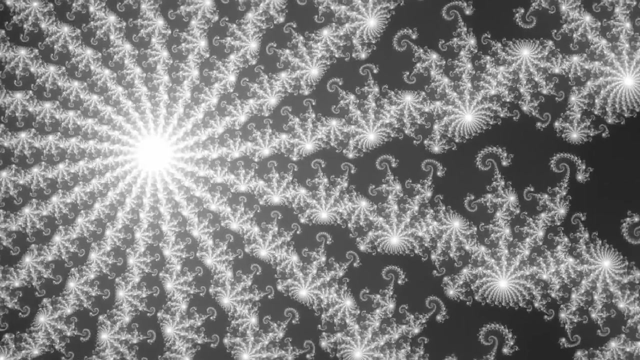 we can use this shader to quickly visualize the variety of shapes offered by the Julia set when we vary the constant C. Despite all these advantages, I decided to stick to the CPU because double precision compute is either not supported or have terrible performance on most GPUs. 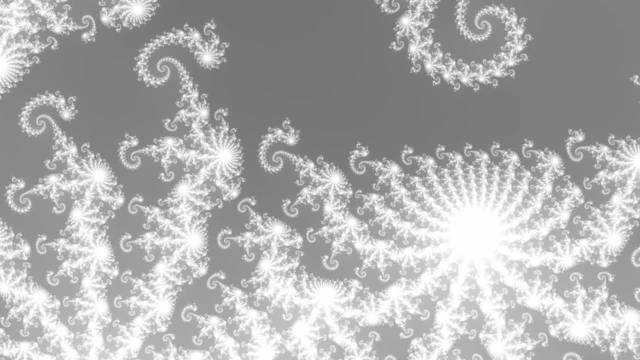 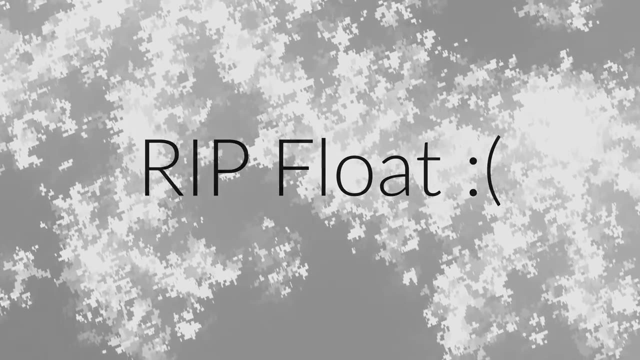 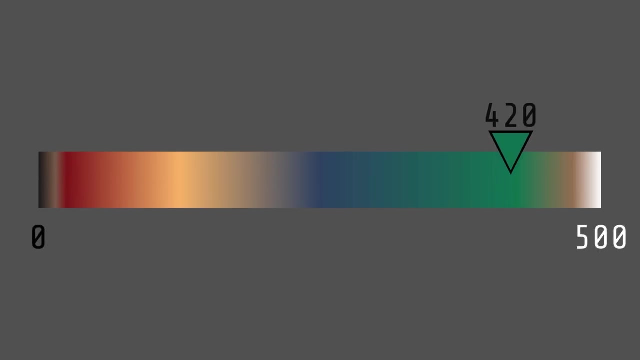 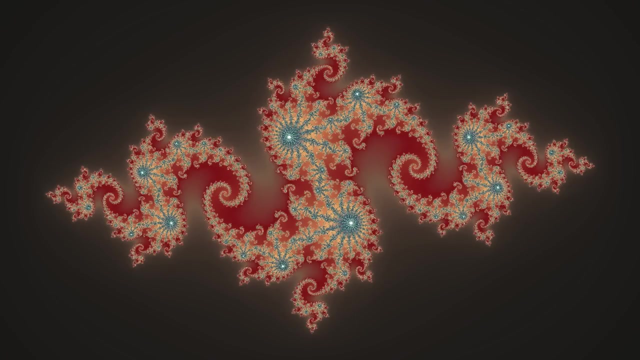 And with simple precision float, the maximum zoom is quite low. So far, we've only used a simple gradient to compute pixels colors, but we could use a multicolor gradient instead, Despite the fact that we are rendering our fractal with high definition. 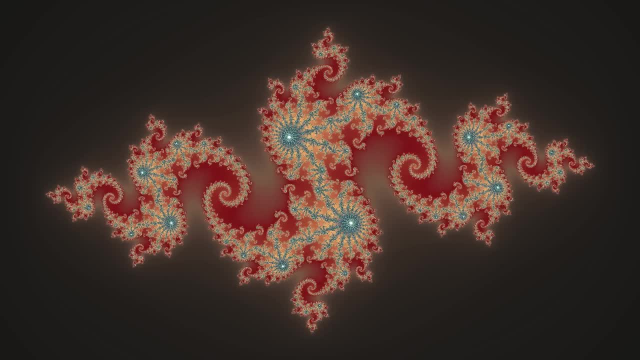 it contains a lot of aliasing. This is to be expected because, by nature, fractals contain unlimited amount of details, unlike our screens and their finite numbers of discrete pixels. Fortunately, we can mitigate this very easily, But it won't be free. 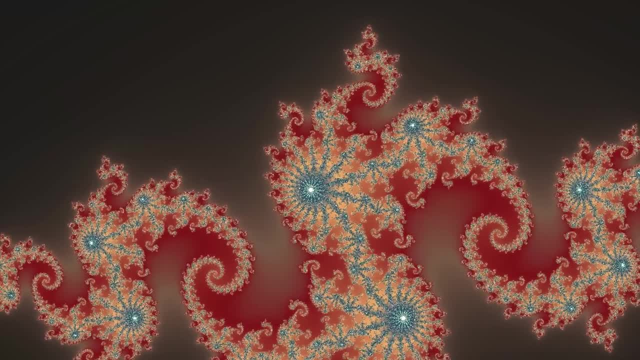 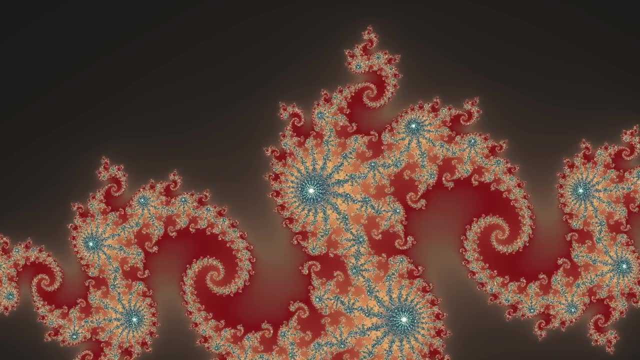 The problem here is that we are strongly limited to the number of pixels that we have. We are strongly subsampling the fractal by computing the color of each pixel And because of this the correlation between pixels' colors is very low in some areas. 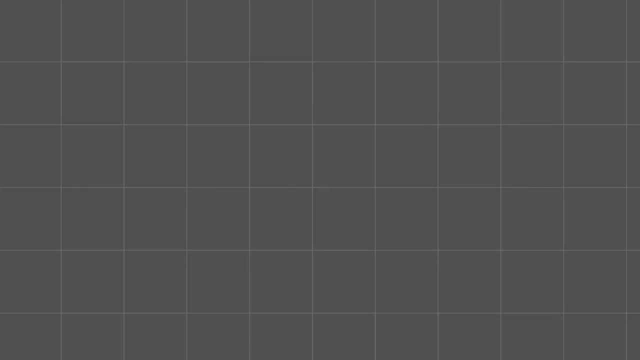 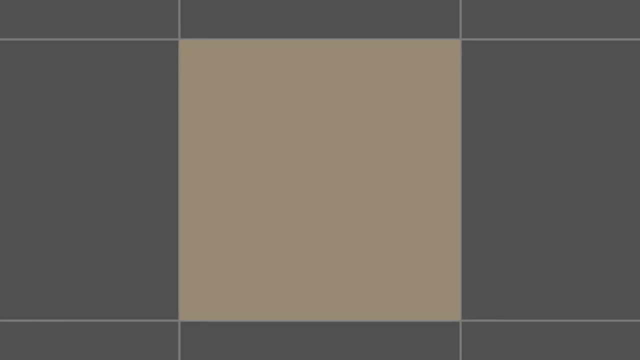 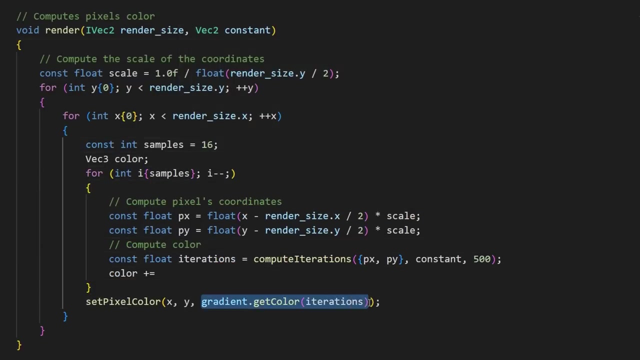 To help with this, we can simply average multiple samples for each pixel instead of just considering the point at its center. The obvious downside of this approach is that it multiplies the time required to render a pixel by the number of samples. So if we want to render a pixel by the number of samples, 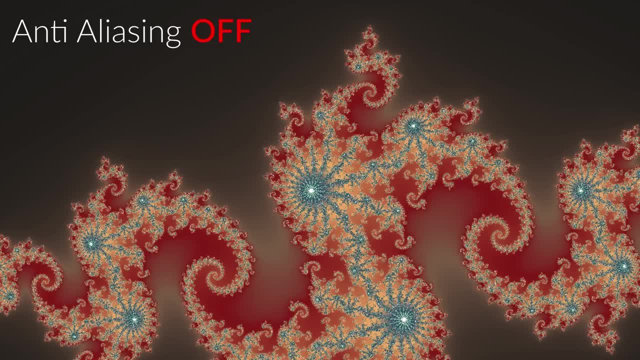 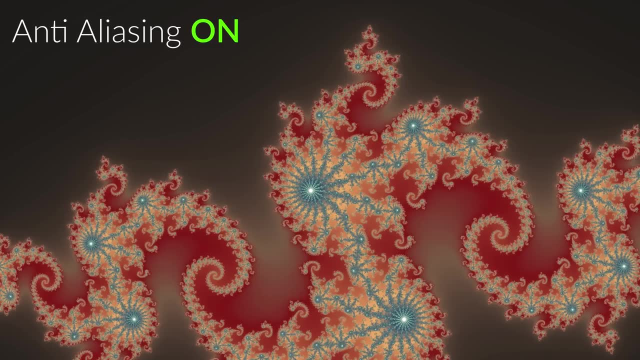 we have to use a very simple method. We can use a very simple method and we can also use a very simple method to render a pixel. by the number of samples we have, The image is now looking much better, but is also 16 times slower to render. 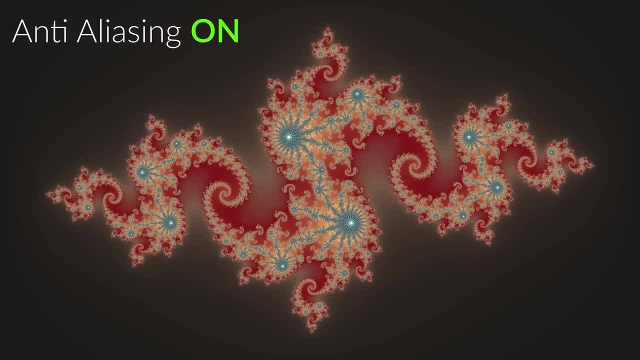 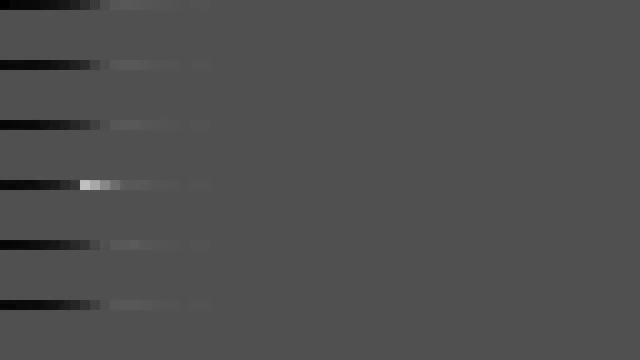 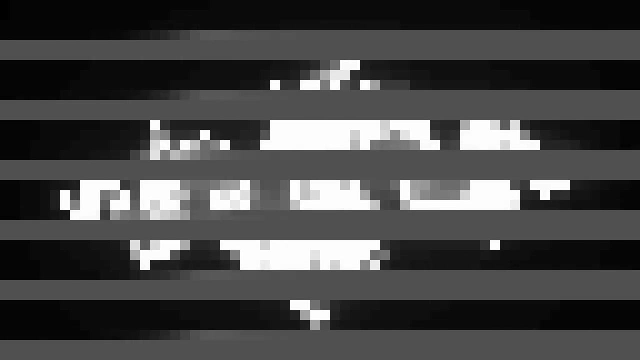 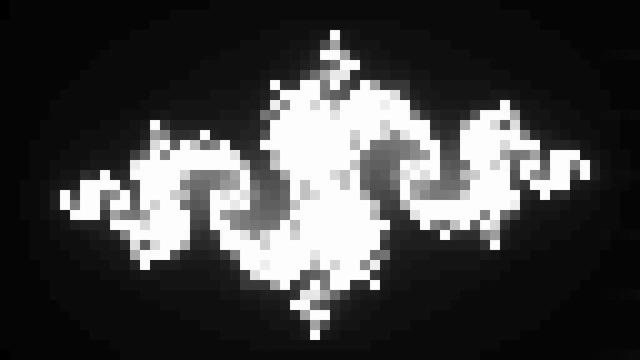 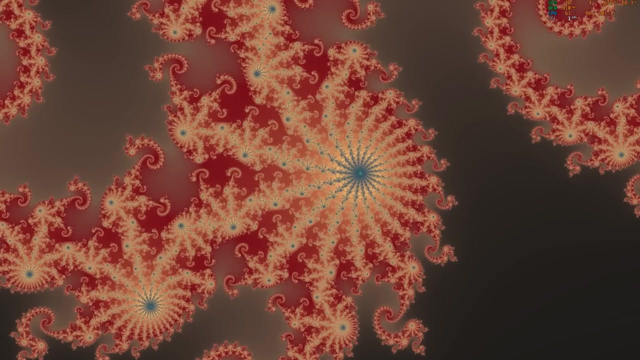 Thankfully, rendering is often very easy to parallelize, and this one is no exception. To mitigate the effect of the supersampling, we can use several threads To compute pixel color in parallel. Even with multithreaded rendering, the time required to render a frame is way higher than a few milliseconds. 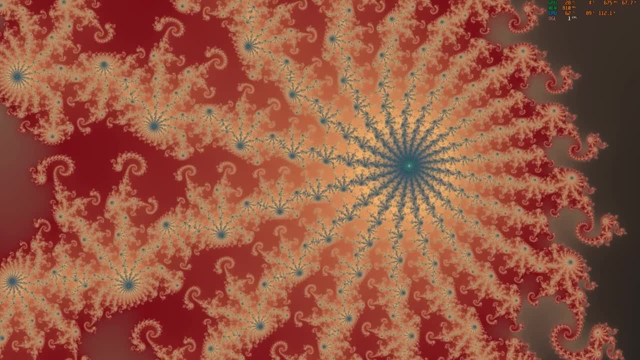 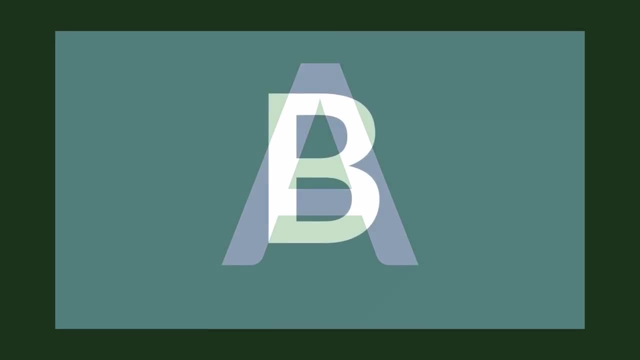 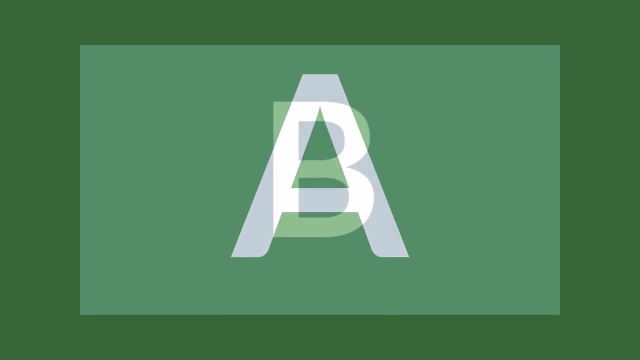 A trick that can be used to perform fluid navigation is to have the next frame being rendered in the background while the current one is still there. The initial frame is displayed and transform according to the camera, And here is the result. It is not magic. 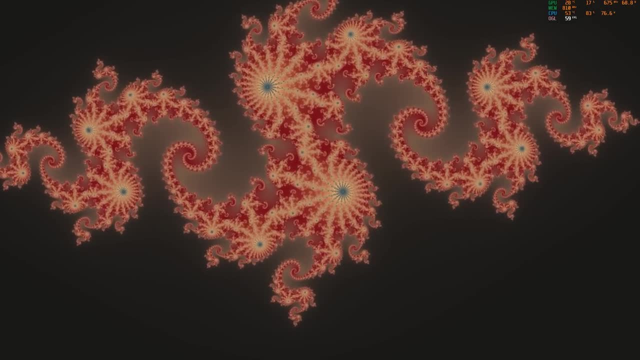 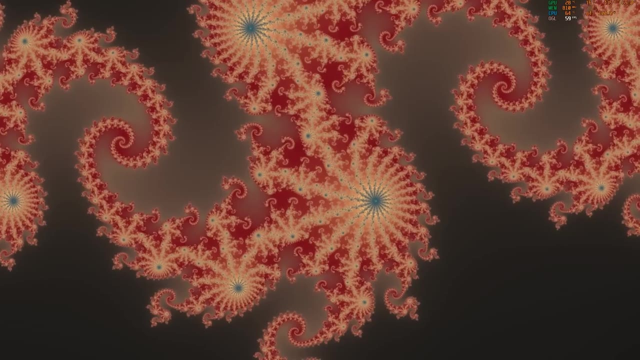 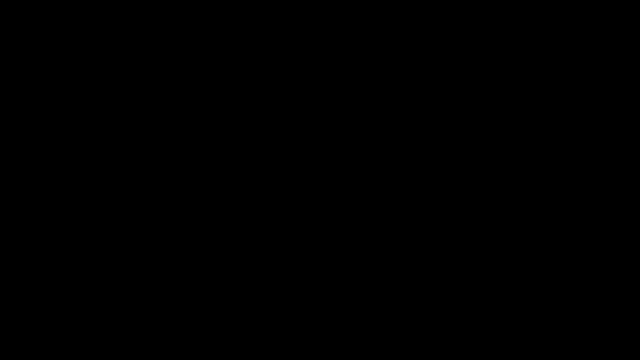 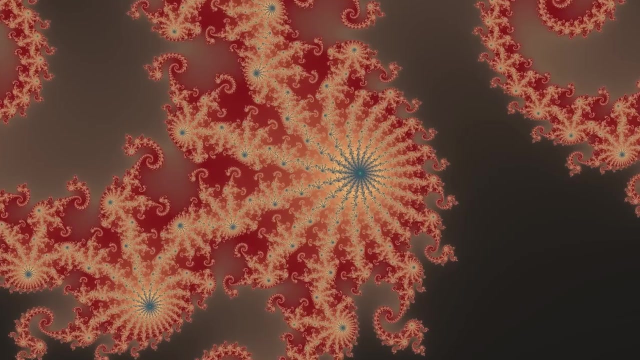 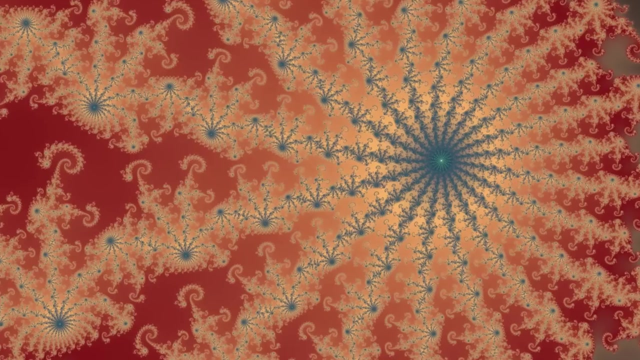 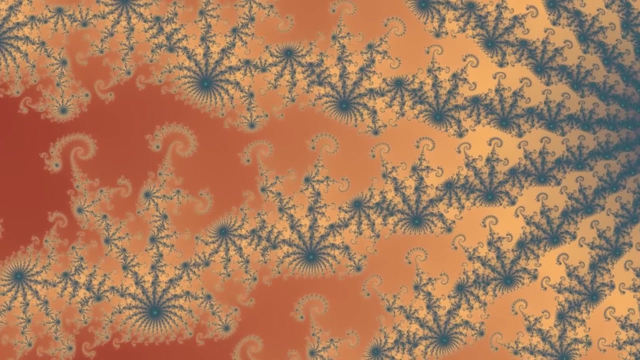 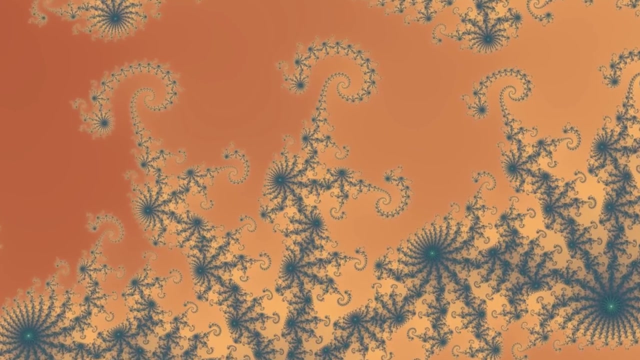 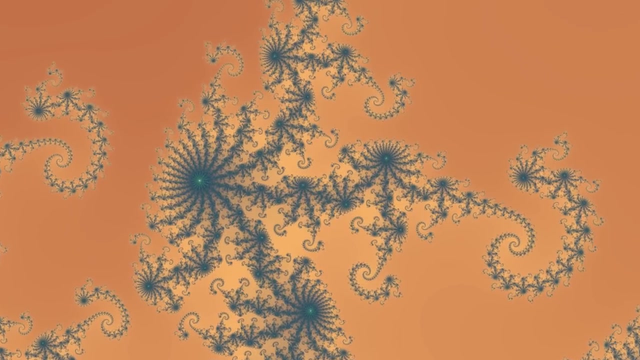 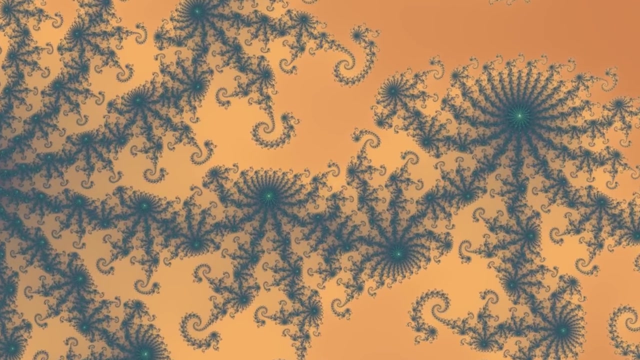 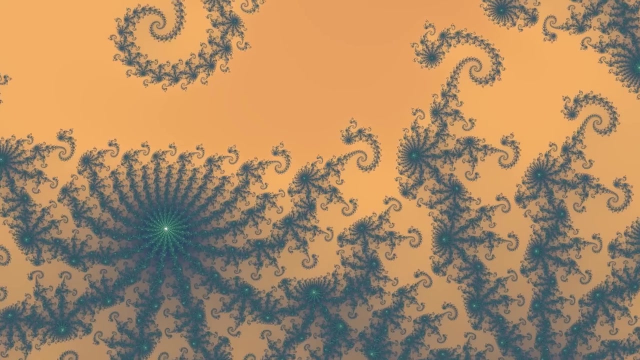 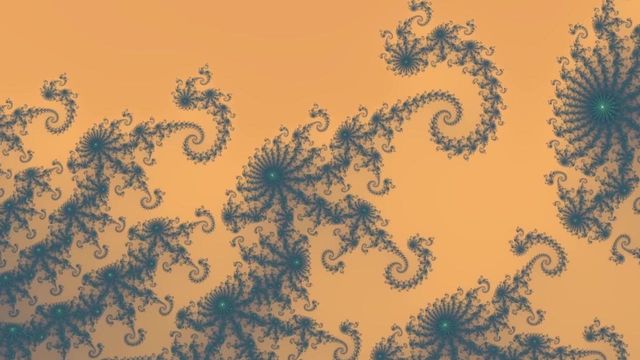 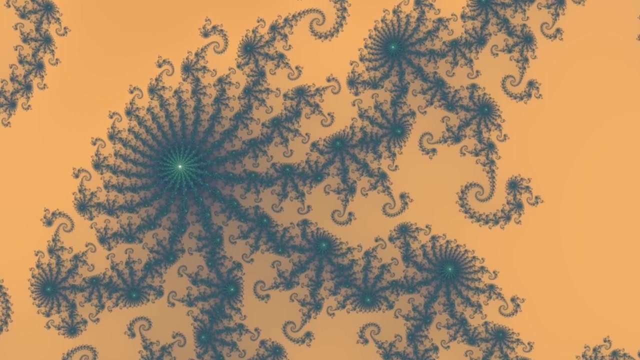 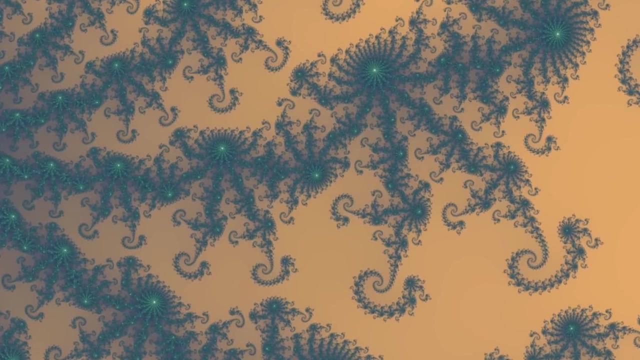 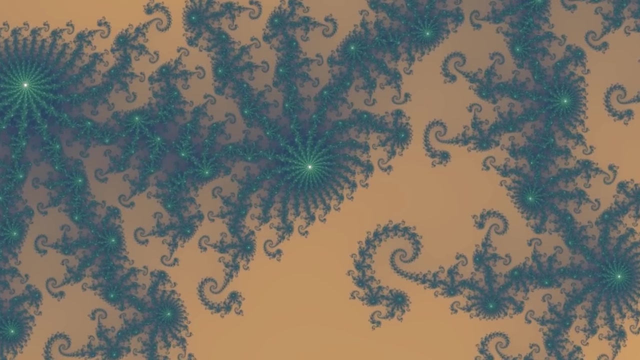 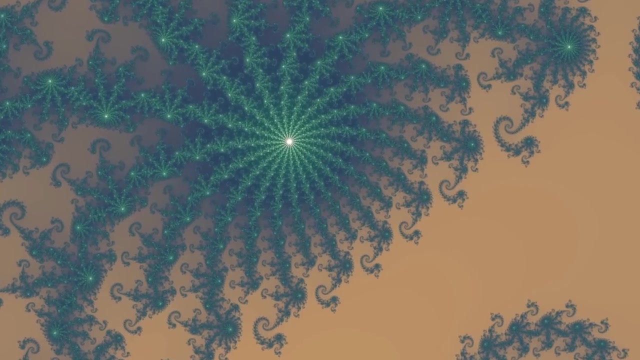 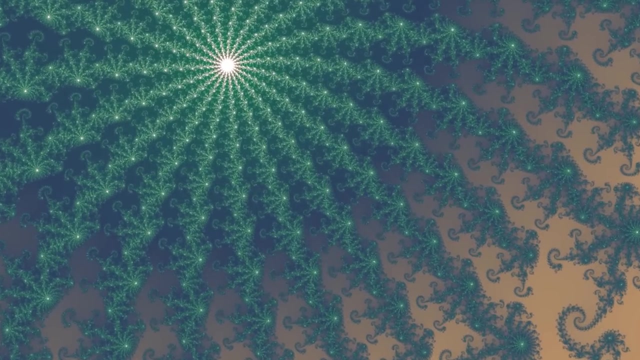 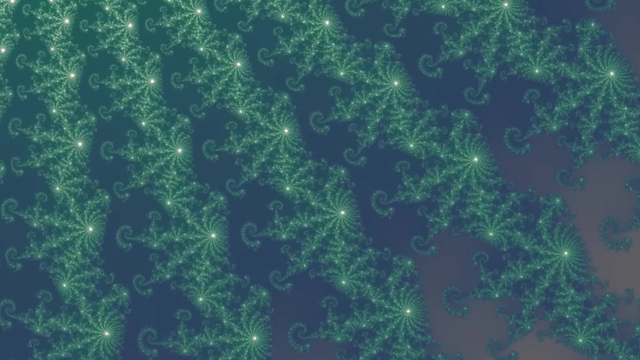 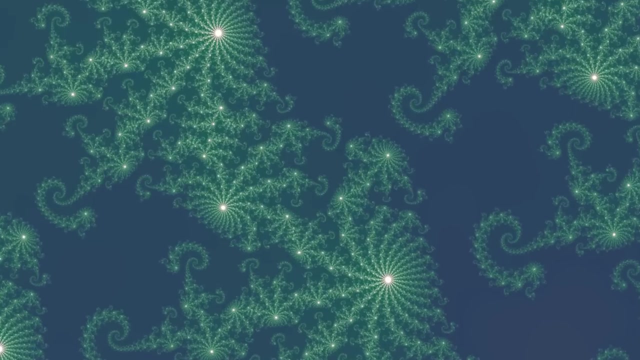 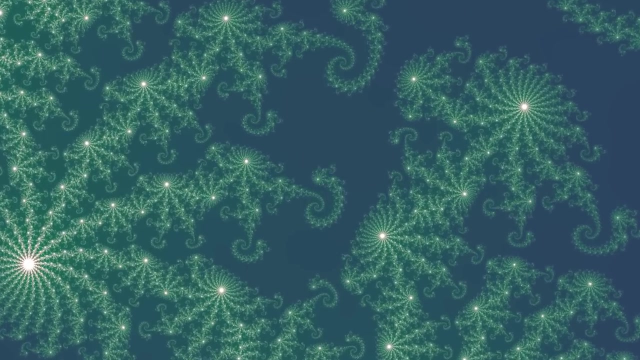 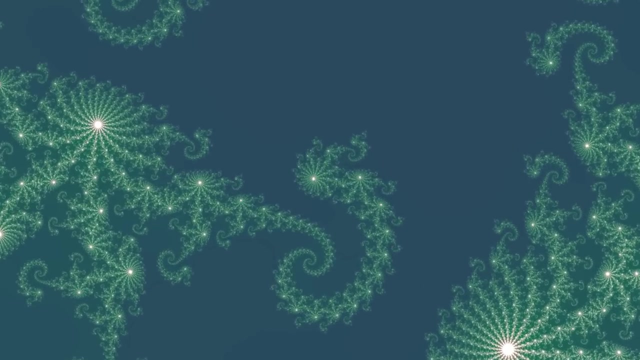 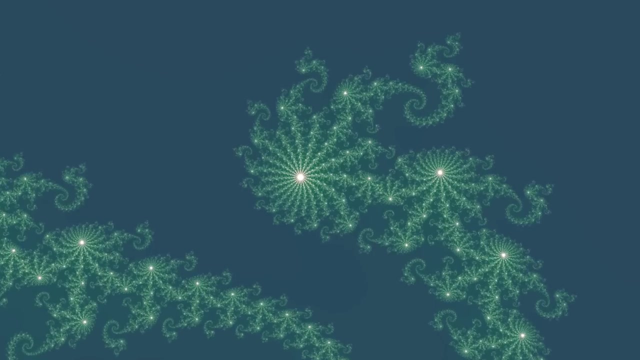 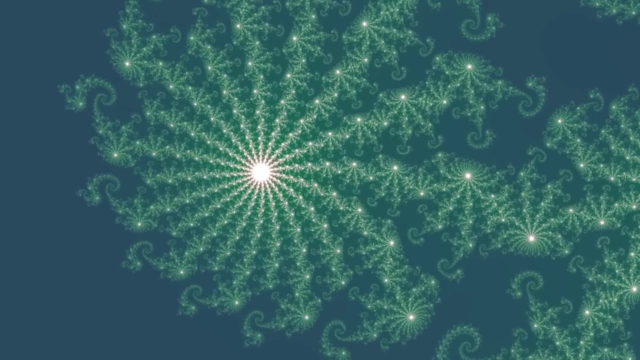 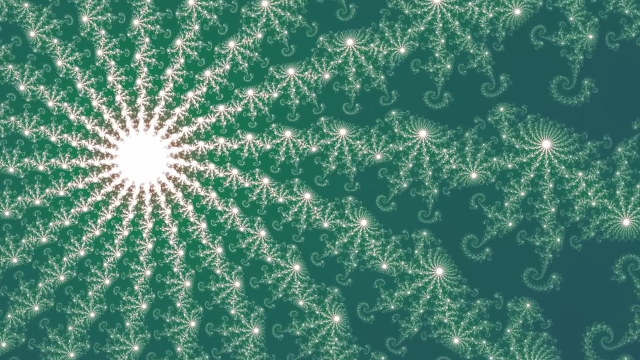 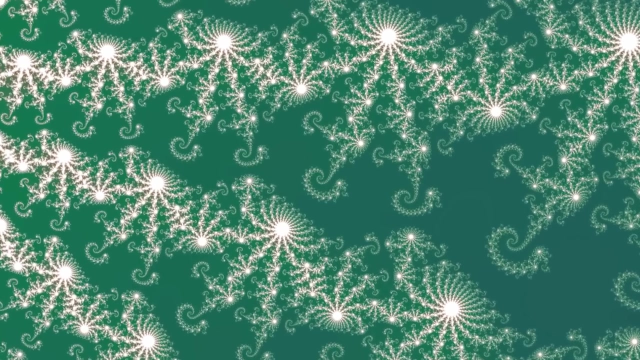 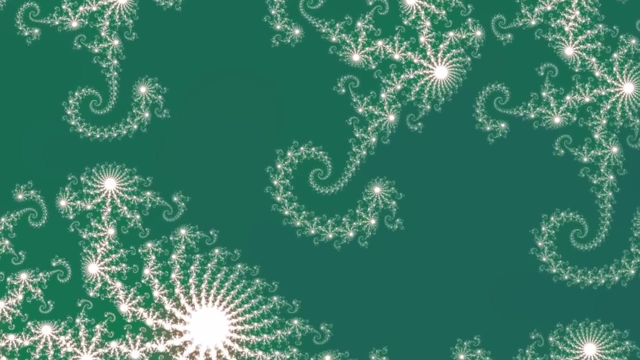 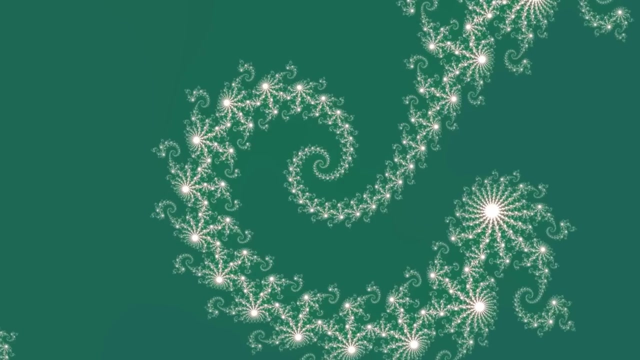 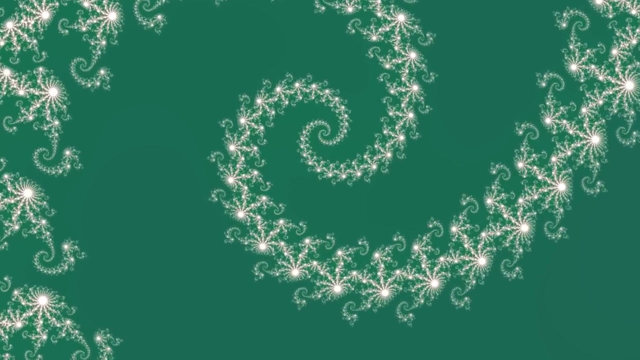 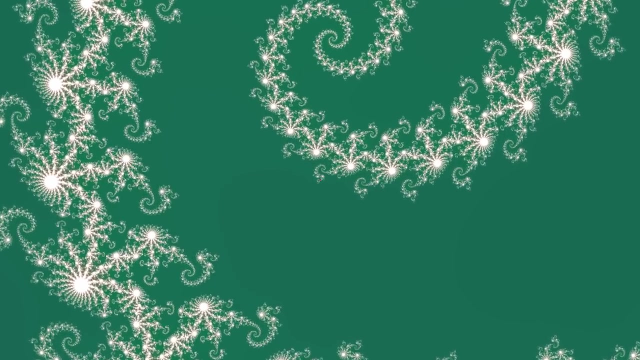 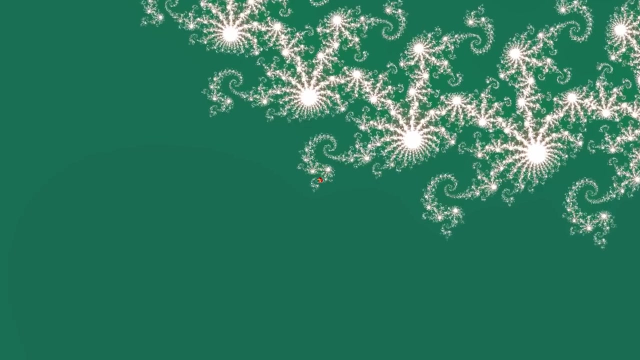 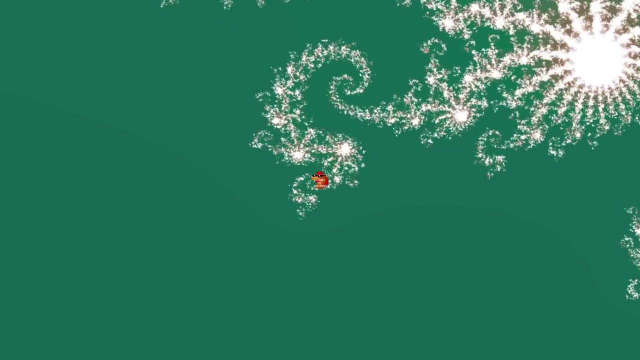 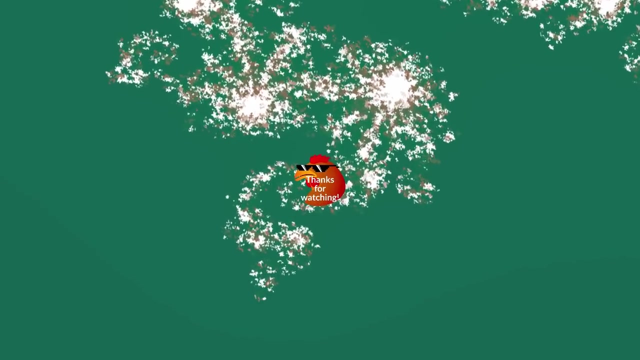 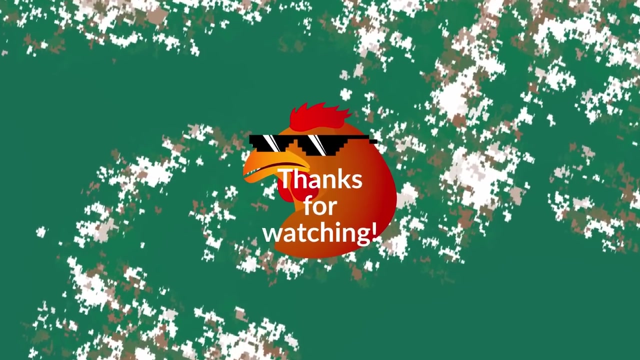